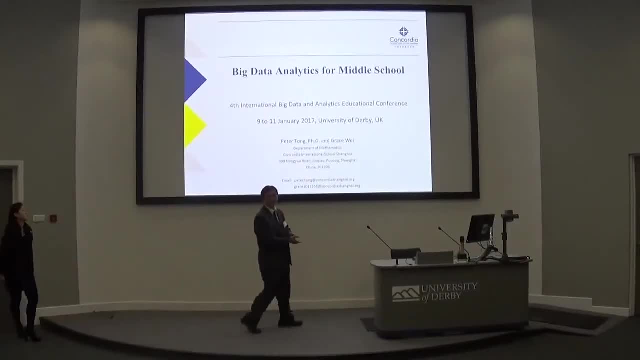 So good afternoon. Thank you very much for attending our talk presentation on big data for middle school. So just a brief intro of what it's about. I've been teaching a big data high school for the past three years And in the past year or so we see that there's a need to start expanding big data to middle school there. 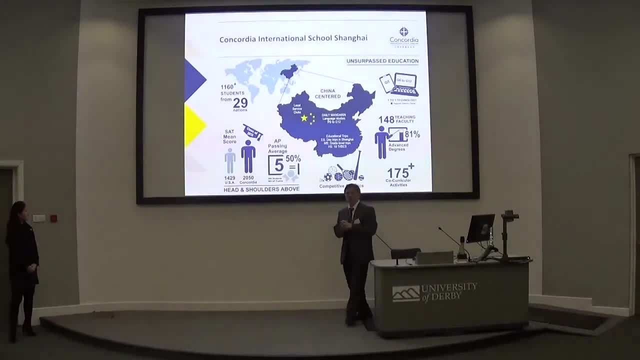 Now just a very brief intro of Kofuni International School, Shanghai. So we actually located in China itself And these are some of our statistics. on our school. We run the American program. We have about 1160 students, about 148 teaching faculty. 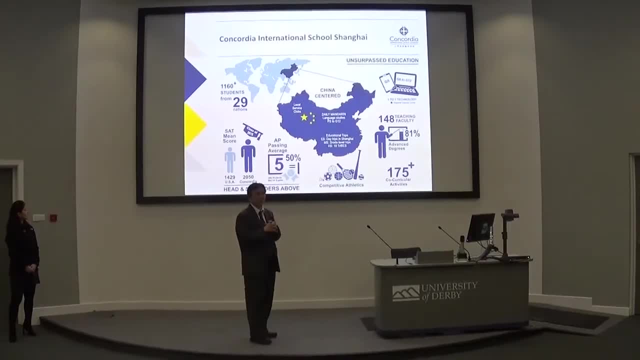 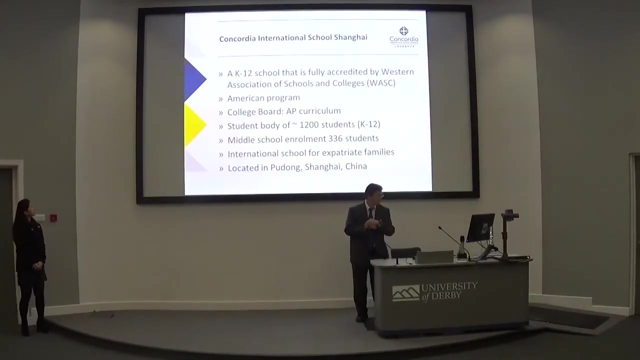 and one-to-one computer from grade 5 and grade 6 to 12.. But basically an international school that's catered for the expatriate community located in China. So this is just a little bit more about what the school is about. 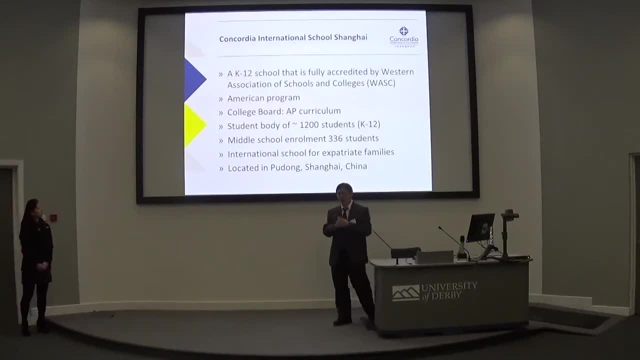 And, without further ado, I'm going to introduce Grace Wei, who helped me to develop the program for big data for middle school. Grace, Good afternoon everyone. I'm Grace. I'm currently a senior at Concordia International School, Shanghai. 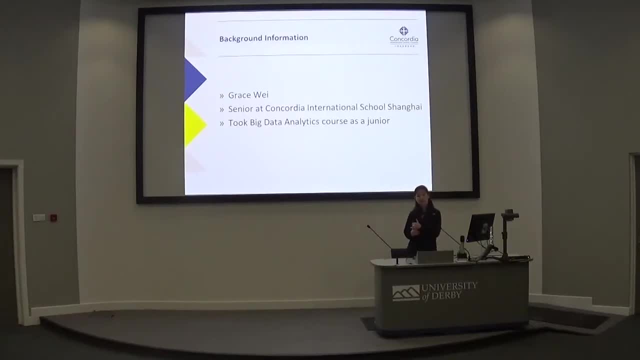 I took the big data analytics course last year as a junior And before taking the course I had absolutely no idea what big data is. But after a semester I feel like I found a new interest, or I can't even call it as a new passion. 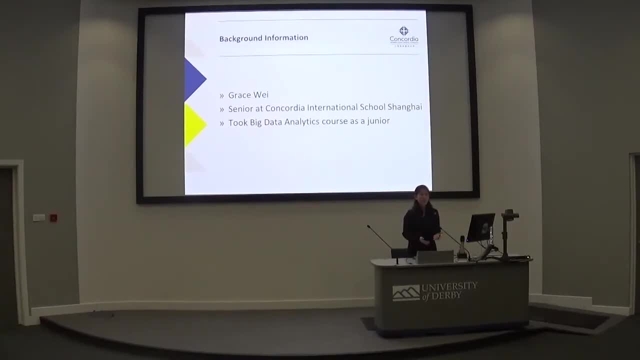 I'm particularly fascinated by how powerful big data is, by how just mere numbers can have such an impactful influence on myself and the world, How it can change lives, how it can save lives and how it can give us so much more time. 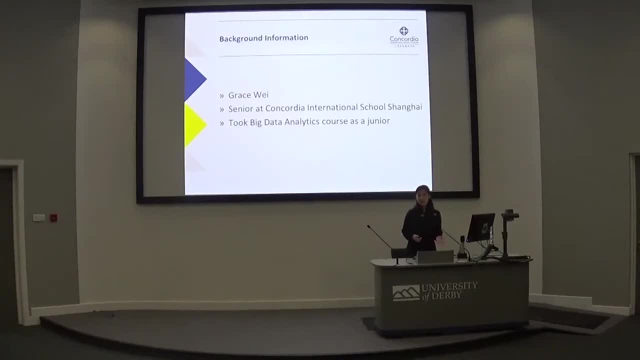 And other than big data, my other interest is education And luckily, Dr Tong has given me this golden opportunity to combine my two interests in this project, which is developing a big data course for middle school students, And I'm so honored to be standing here today. 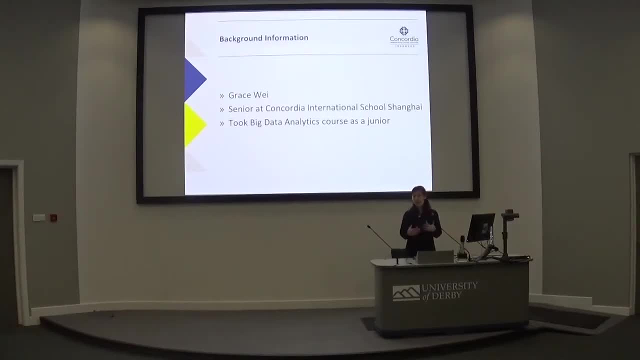 and sharing with you about some information about this course. And let's get started. So first I'm going to answer this fundamental question of why are we promoting this course? and there are mainly five reasons. The first one is we want to stress about the importance of computer or computational literacy in our lives. 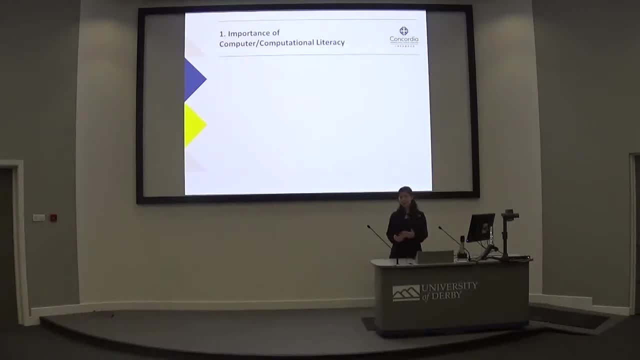 Technology is important, as we have all recognized already. It is relevant to every field, And thus we just want to let the middle school students to be able to have the opportunity to have the A experience in getting in touch with these elements, And so no matter what discipline the students go into, 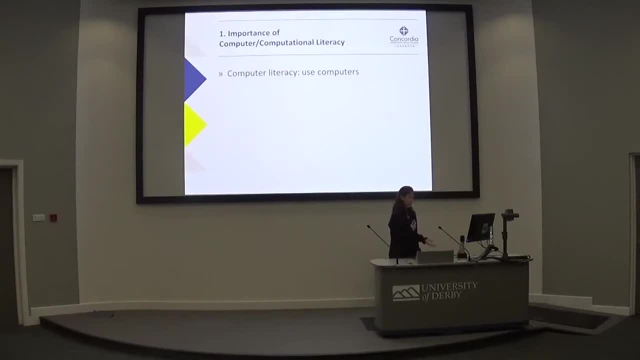 some training in computer or computational literacy is going to be helpful, And here computer literacy refers to the ability to be able to use computers, And computational literacy refers to the ability for students to be able to solve problems using computational technologies, And which requires students to know some level of programming. 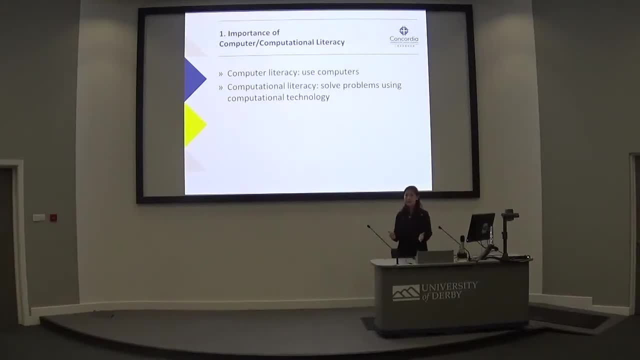 but it can range from just running a simple Excel formula to running an entire elaborate computer system, And in this course the students will be studying how to use these three softwares: Tableau, Excel and IBM Watson Analytics. These three softwares will let them be more familiar with how to use computers. 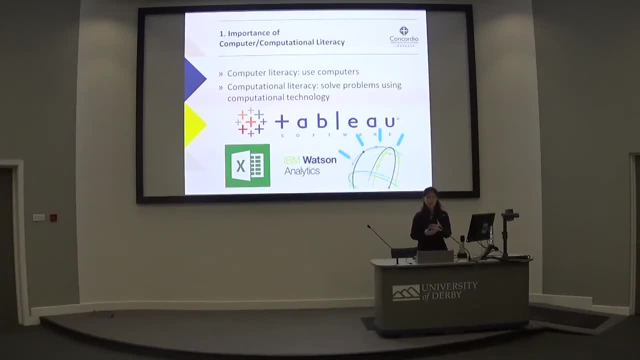 for like a more legitimate reason other than just programming or having fun, I'm sorry, other than just having like gaming and then YouTube videos, And also it will be helpful in your later lives too. The second reason is what I am most appreciative of. 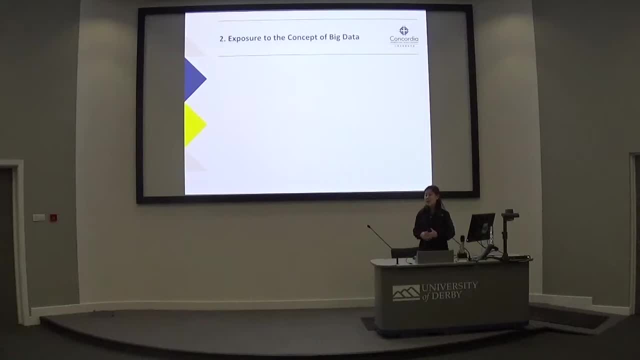 I'm very appreciative, after taking the course myself. It's being exposed to this concept of big data. Big data is relevant to all fields And it has become an important tool when it comes to this decision-making process. Insurance companies use big data to evaluate a person's credibility. 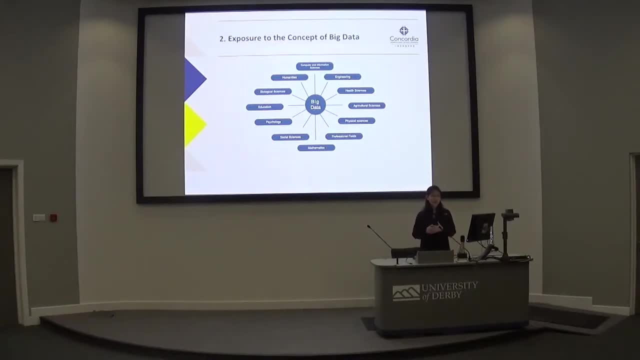 Or retailers are being able. sorry, retailers can optimize their stock based on the predictions generated from social media data, Or personal smartwatches or bracelets are collecting personal data that can be later used to analyze disease patterns. It has transformed how we live, think and work. 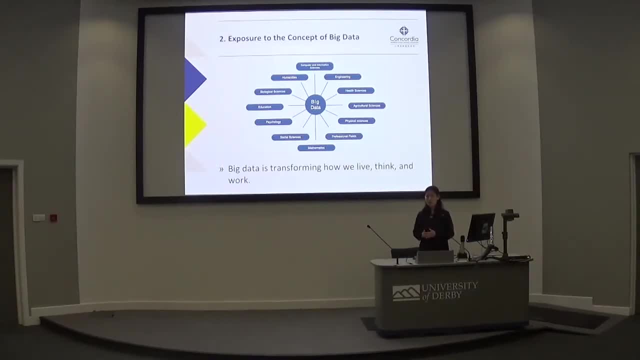 So it is not only important for the current generation to know the importance of big data, but more importantly than for the younger generation to be exposed, Because they will be the ones who are more influenced by this idea as this big data technology advances. 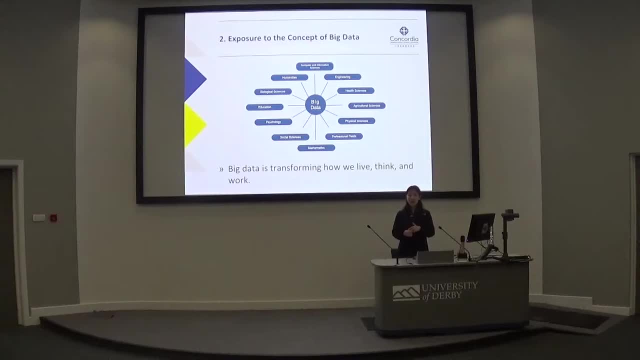 And from my personal experience, I also feel like, after learning about this subject, I am more knowledgeable as a person in this society, because I know more about each field that is related to preparing examples how this operates. It has made me realize how the world makes sense. 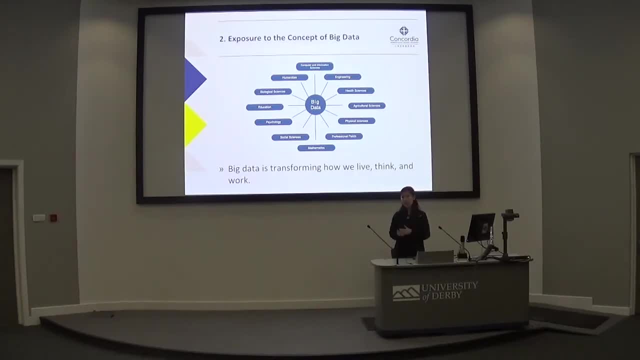 And I really wish that the middle school students are able to have this opportunity to feel what I have felt even earlier at this stage. Being exposed to this concept will let them learn more about themselves. They can explore their own interests because the design of the quarter school 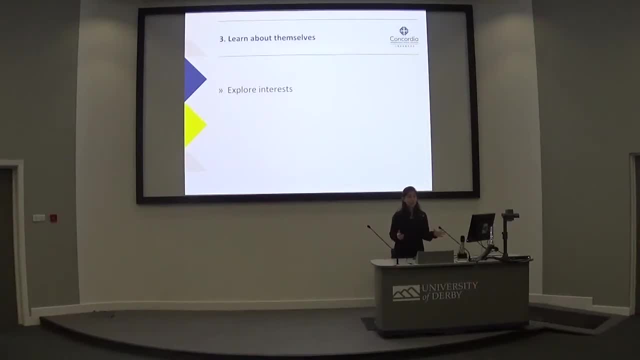 allows students to have this chance to combine their interests with the skills they learn in this class And to generate something that they really care about And because they will be doing this self-directed project later as a final or major section of this course. Also, maybe they can discover new passions, just as I did. 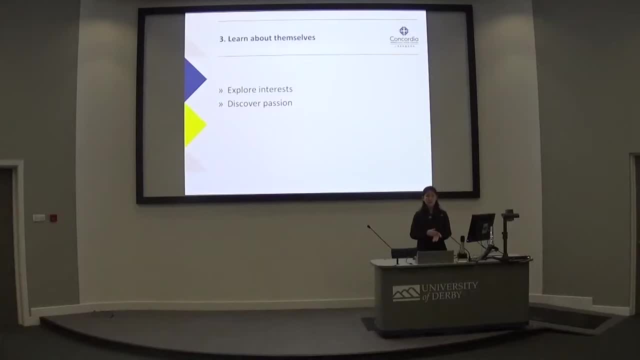 Because this is going to be a new field that the middle school students are being exposed to. Maybe they will find interest in this field as well, So it will provide more choices of careers for them, as big data has a lot of other job titles as well. 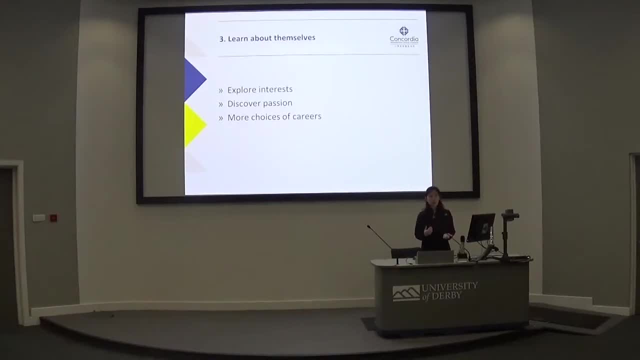 And also it will let them know more about themselves, as in what are their strengths, what are their weaknesses, and also what they really enjoy doing or what they don't enjoy as much. The fourth reason is to fulfill your goals. The fourth reason is to fulfill the demand of big data scientists. 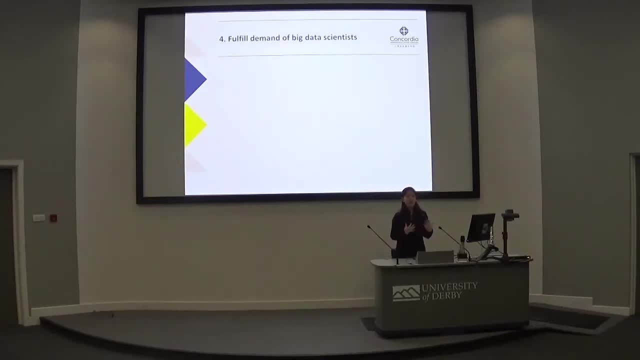 As we know that there's a lack of data scientists in the world in the job market right now, But it is predicted that by 2018, there will be at least one million data scientists needed, Which universities or high schools or professional schools. 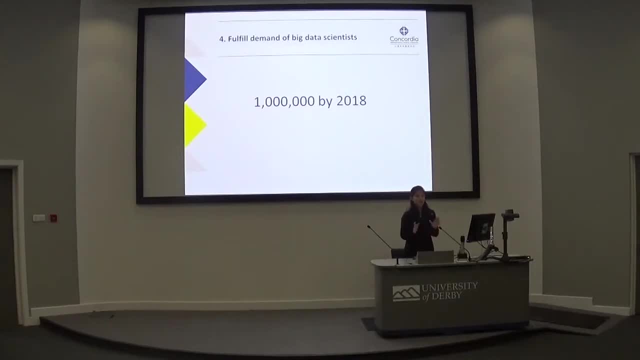 are not training them fast enough. So maybe starting with the middle school students can help to reach this goal, So they can do it sooner and just benefit the world as a whole. The final reason is to meet the purpose of middle school. 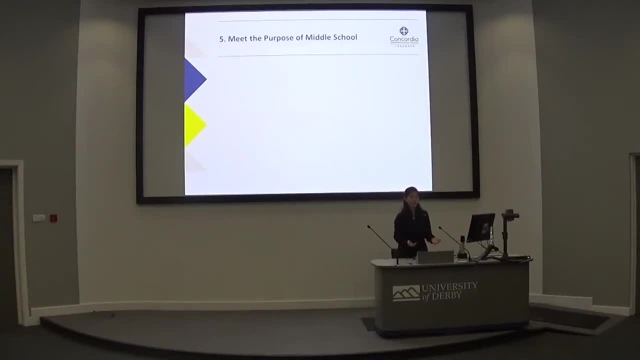 Middle school is not just about learning grammar, learning mathematics, learning history, learning about science. It is a person's transition from being a children to being a child, to being a teenager, And it is often the stage where they are questioning or discovering. 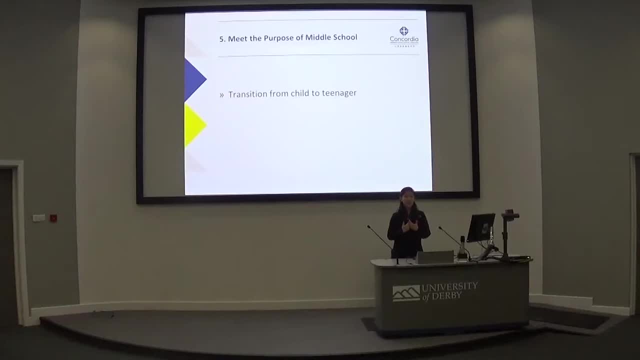 or wondering about their passions and their personality. So, other than knowing who they are, it is also a time when they start to learn important life skills, Such as learning to research, learning to think critically and also to being able to analyze things. 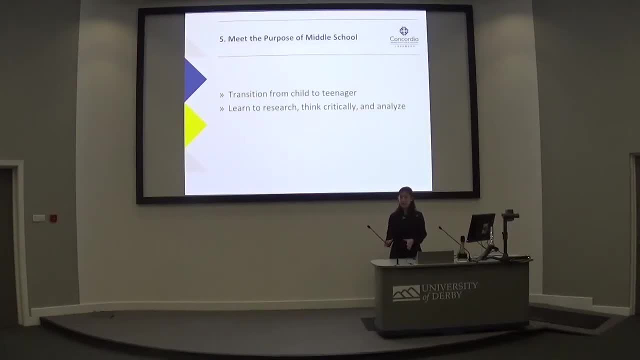 Which are all important qualities in this big data subject. Also, they will be able to learn how to be a better team player And they can be more creative, because big data needs them to think, maybe sometimes outside of the box, to find a correct correlation. 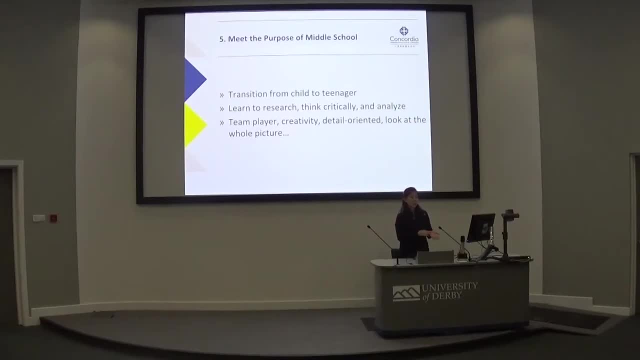 And they will learn to be more detail-oriented, as well as being able to look at the whole picture instead of just focusing on one point. Another important part about middle school is that it is a time when students are encouraged to be a part of the society. 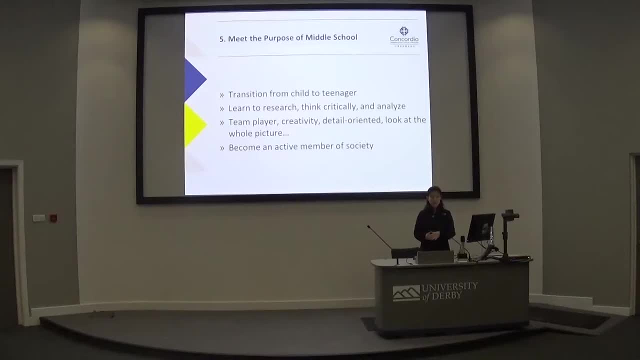 And this course can be their first step, because it is when they will be in touch with the world, knowing what is happening outside of their own family and their own school community, And they will just get a more general sense of what is it like out in the real world. 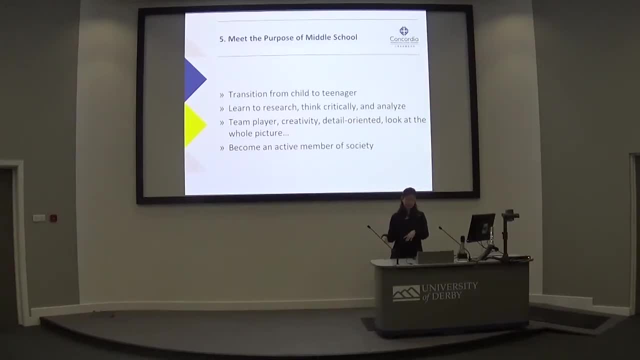 And it is just going to be a bridge for them to connect them with the outside world. Well, some people may say that middle school students are too young to understand this concept, And I will say no to this question, because the course will be taught in a very detailed way. 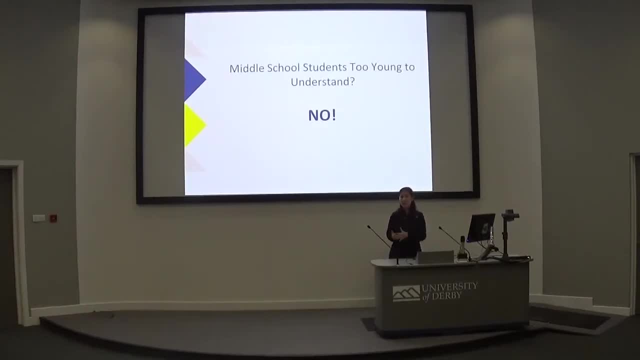 and also in a very in a pace that will be suitable for middle school students. So this course will be an elective, which means that the students who are enrolling in this class will at least be interested in this subject, And it is a 60-minute class for one semester. 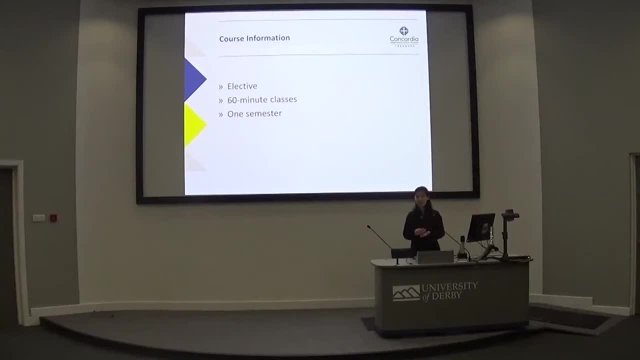 which means that probably about 45 to 50 classes And it you know, and the key about this course is not to enforce them to learn about skills that critically, but more for them to promote interest and more for them to explore new things. 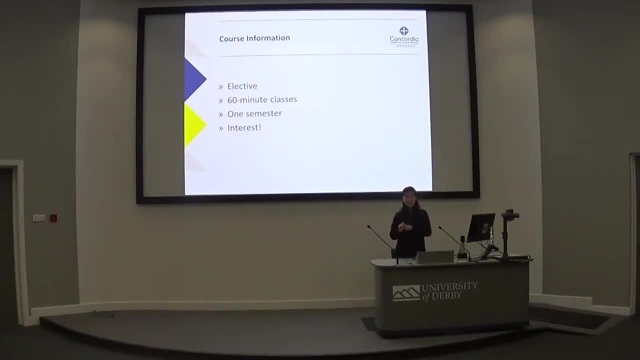 And one key thing about this course is that it is really hard to find resources because, as we all know, there is no textbook for middle school students about big data. So this course, that is a major challenge. but because of internet and how many resources there are online, 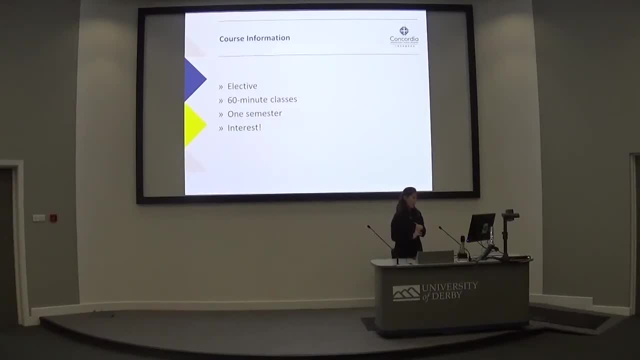 so this course can be still implemented. And the final one is that this course will be divided into five parts, shown in this graph, And I will be I'll go into more detail about each part. The first part, of course, is going to be the introduction. 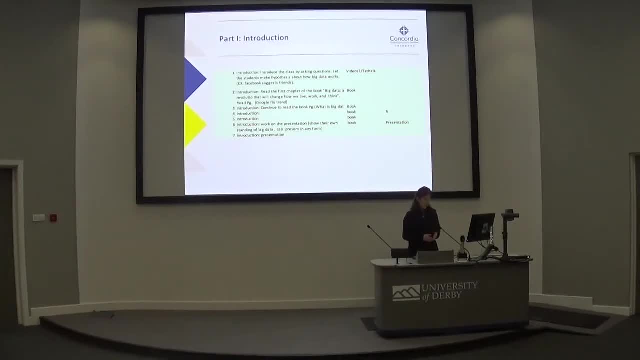 And it's going to take approximately seven classes, And this this section will be answering questions such as what is big data? And also about how is big data used in our lives, as well as the risks of big data. We cannot only stress about the benefits of one thing. 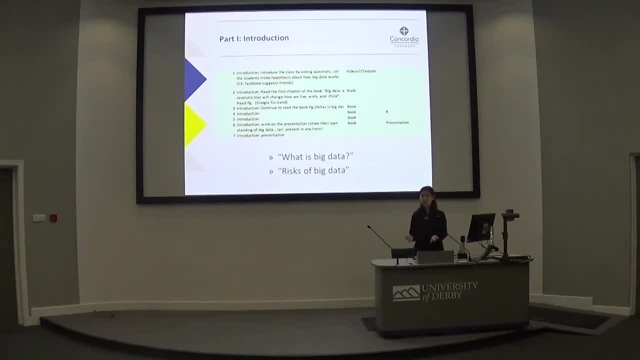 but we have to look at both sides, especially for younger kids, so they will not be misdirected in later life. And the introduction: at the end of the introduction, the students will be presented on what they have learned. They will be reflecting on what they learned as they. 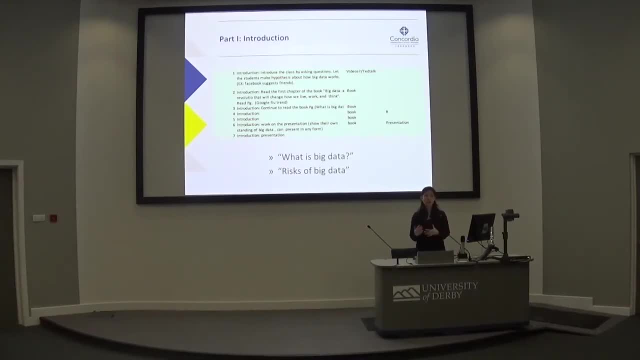 as maybe like a new subject, and also: what are their future goals? what are they looking forward to in later classes? It was a. it can be an opportunity for students to tell the teachers what do they look forward to? The resources for part one will be this book. 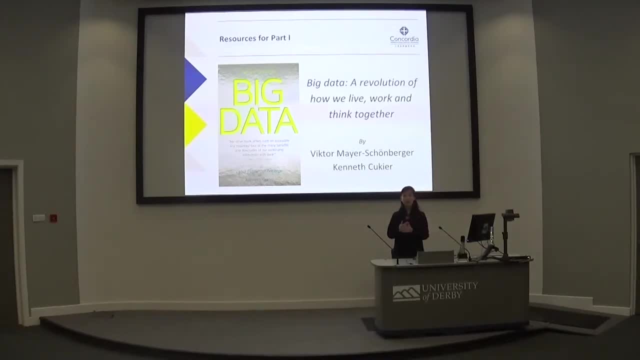 Big Data: a revolution of how we live, think how we work, live, work and think together by Victor Mayer Schoenberger. and he needs to keep here. sorry, I don't know how to pronounce your names properly. 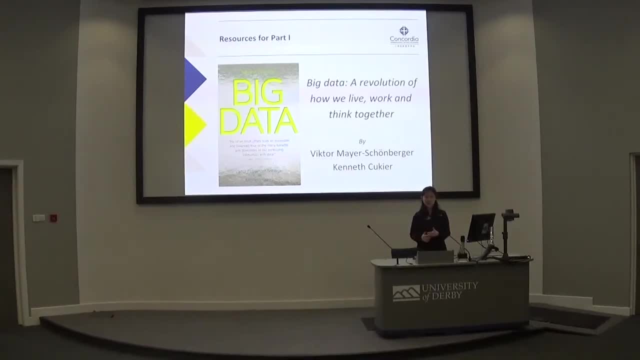 But this is the textbook that the high school course has used last year, at least for my year. I really enjoyed reading the book because it has given so many great examples and the language is very simple And very direct. So for us, 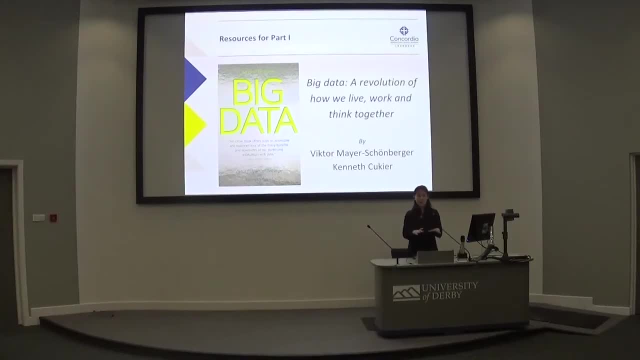 we, each student, was responsible for one chapter and we became the teacher and taught and shared our information with the class. But it's going to be different with the middle school students, as they don't quite have the ability, that strong ability. 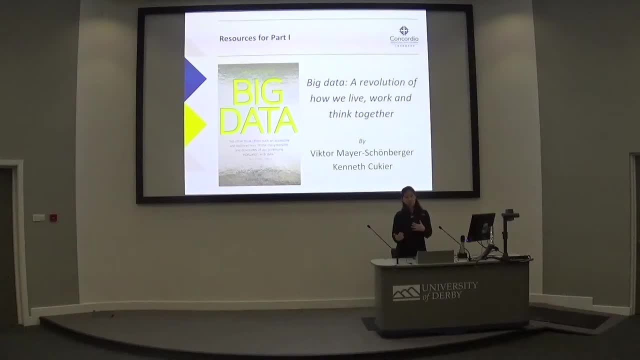 to carry on the class. So the teacher will be the director and then they will be. I don't think they will be reading the entire book, but they will be focusing on the book. they will be focusing on the first chapter, where it's the introduction. 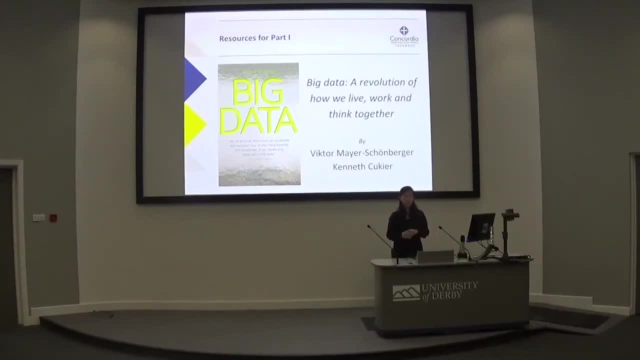 and telling them general sense of what is big data, and also the seventh chapter, which is about the risks of big data. Other than the book, they can also- there are many YouTube videos online that introduce what is big data. that can be used as a hook to the course. 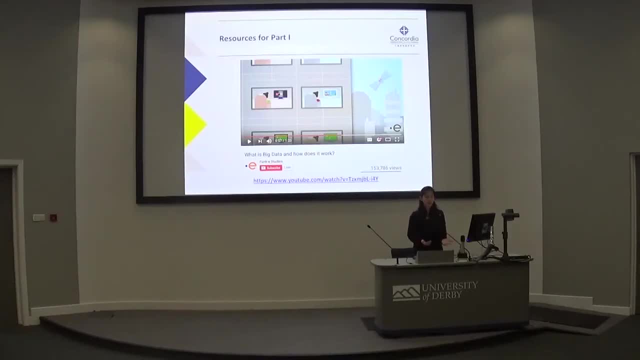 or like a more general. they're giving a more, another review for what is big data. So they're just one example and another example. They have great animation and then the language is simple. of course, Part two will be focusing on showing more examples. 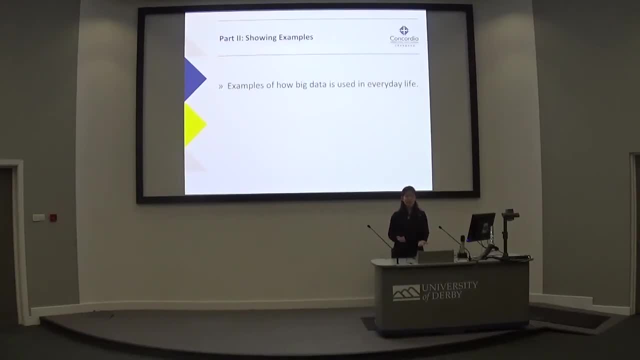 of how big data is used in everyday life. This course, this part, will not be long. it will take approximately five sections, but the key is just to convey the message that big data is in everyday life and it is happening around us. 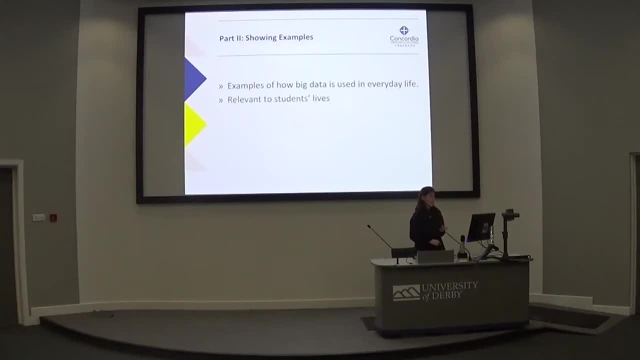 And like this can be achieved by showing examples that is relevant to students' lives, such as examples in social media, gaming or sports, or maybe food as well, And some resources for this is tech talks and YouTube videos such as Amy Webb's. 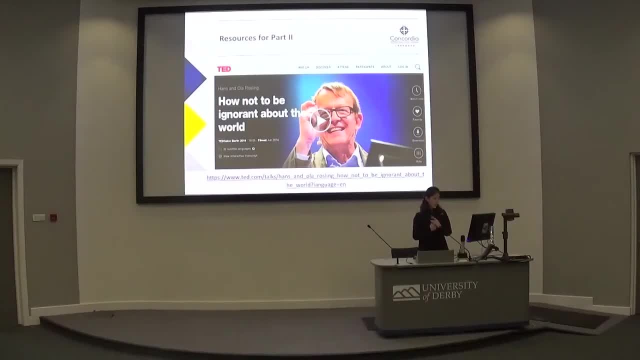 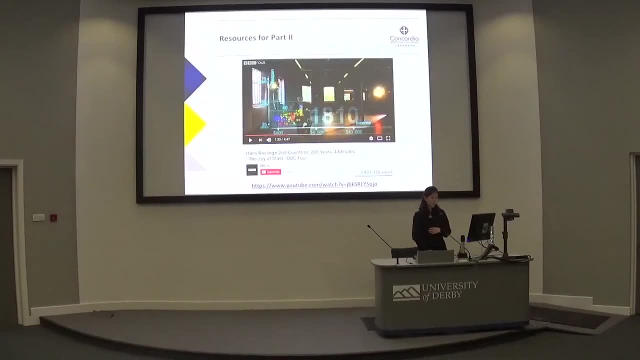 How I Hacked Online Dating and some other stuff, And some of the things that we are going to be talking about are just some of the tools that we are going to be using to help students to learn about how big data is used in everyday life. 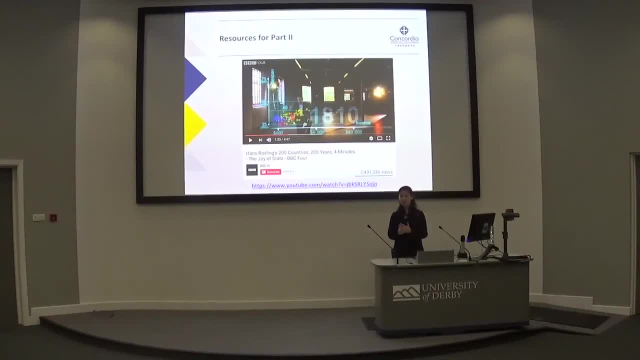 and that's the most important thing, And we're going to be talking about how big data is used in everyday life. So, before I get into the details, I just want to say that I think, that I think, I think we have. 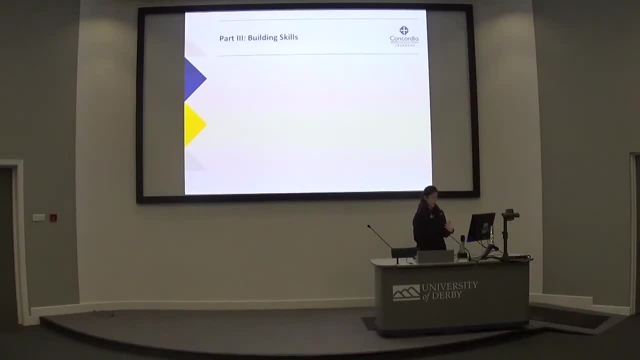 a lot of things that I want to talk about, So I'm going to start with the first thing and then I'm going to talk about how big data is used in everyday life, and they will learn basic skills. So they will be using these three softwares again. 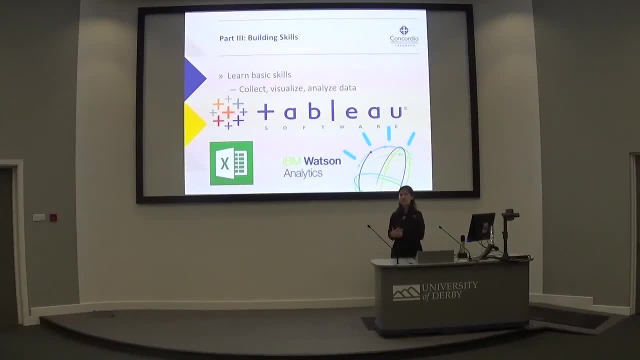 And also they will be learning how to collect, visualize and analyze data. And the analyze part will be the key to in this section. And the tricky part is to find the correct correlation- Correlation- so the teacher will stress about that. correlation does not prove causation. 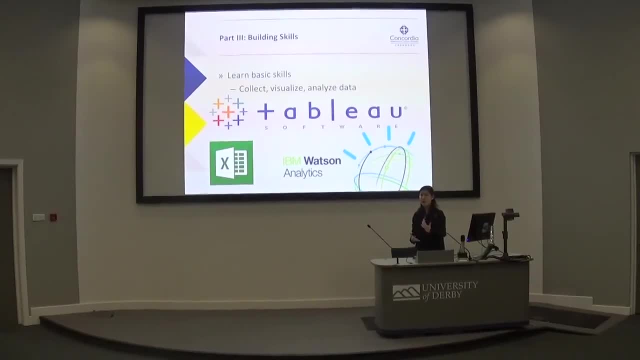 And finding correlation can also help students to strengthen their critical thinking skills and just looking at the whole picture and building the skills that I talked about previously. There are other than these resources. this video, the following of rule two, I think is a great hook to the visualizing data part. 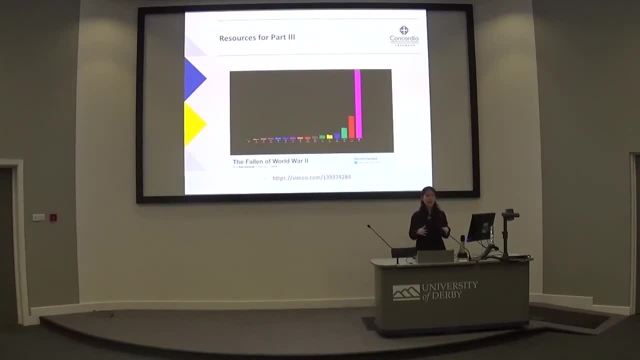 because it has shown the data in a very in a beautiful, informative and illustrative way, And the topic is. I'm pretty sure middle school students have already known about rule two. It's really relevant to what they're learning in their history classes too. 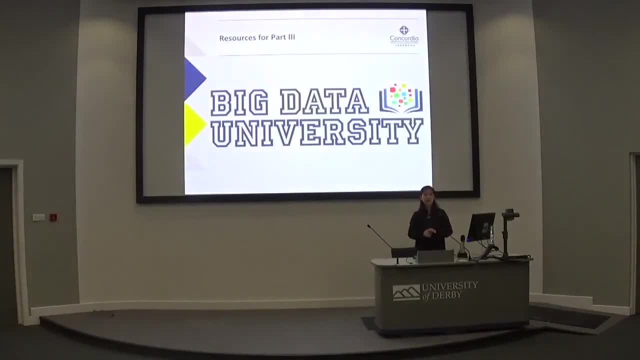 Also, online courses can help with this section, such as Big Data, University Coursera and Data Plus, And the teacher can look more into those and decide how much course they're going to teach. Part four is where the teacher will direct the students. 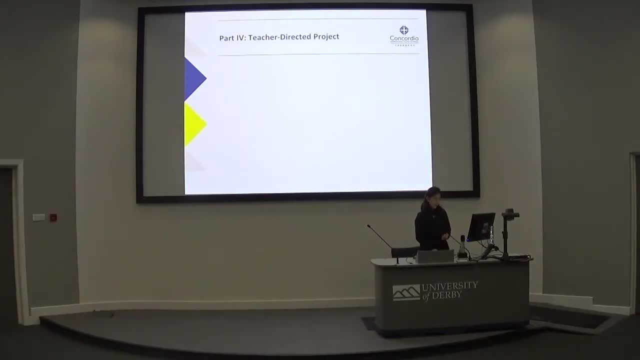 and do maybe one or two projects, So the teacher will guide the students step by step, from collecting, claiming data, to visualizing, to analyzing and to reaching a conclusion all together. Some potential projects for this includes like students can work on how distance from school. 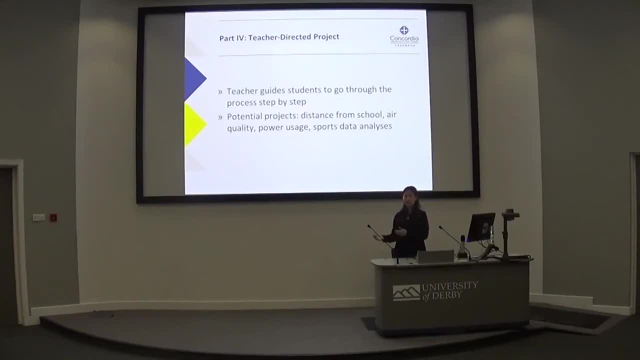 is affected by the school community's division or race or family size or faculties or what sections of the school. And also some other potential projects are like air quality, power usage, sports and also something related to that, Like maybe cafeteria food. 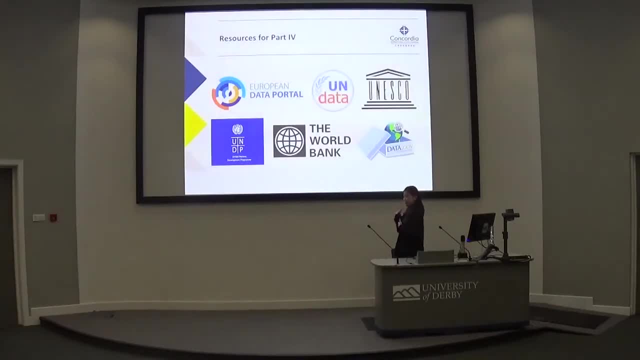 So resources for this is the databases. They can also use data generated from school, And these are just a few very good databases online in their phrase, such as European Data Portal, UNData Datagov, the World Bank, UNDP and UNESCO. 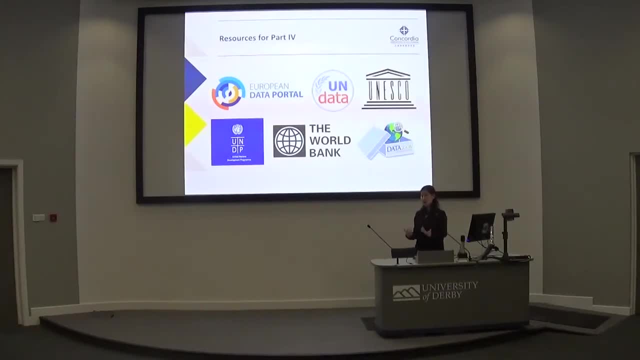 So this for this section: the instructor will be teaching students how to find data from credible sources, And the last part will be the most important part of this course. It will take about 19 classes where students will find their own interests and what they really care about. 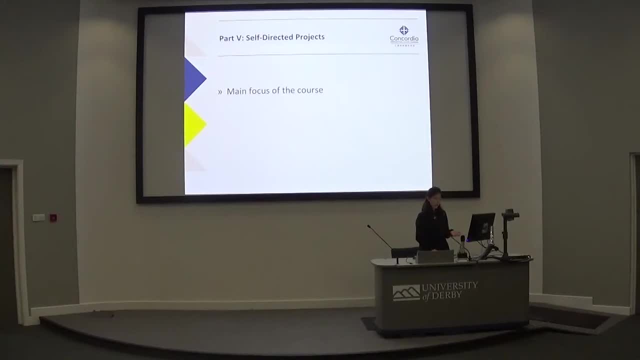 to combine the skills that they've learned to find out what they really care about, What they really want to know too. They will complete the entire process by themselves, maybe individually or with group members, And at the end of this course they will be presenting of what they've learned. 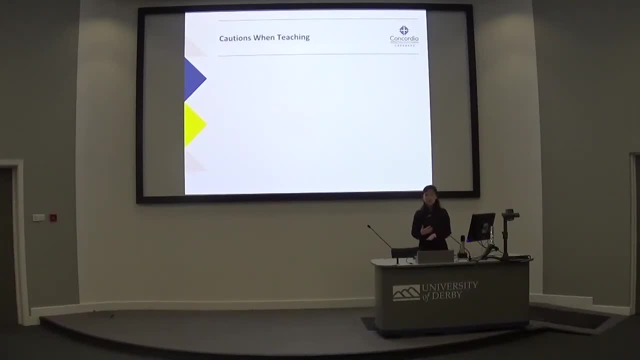 And some cautions with teaching. As I mentioned, big data has many risks. So, other than the privacy issues, I think it is a time when the teacher can focus on telling them that big data is not omnipotent. It's also when we have to appreciate 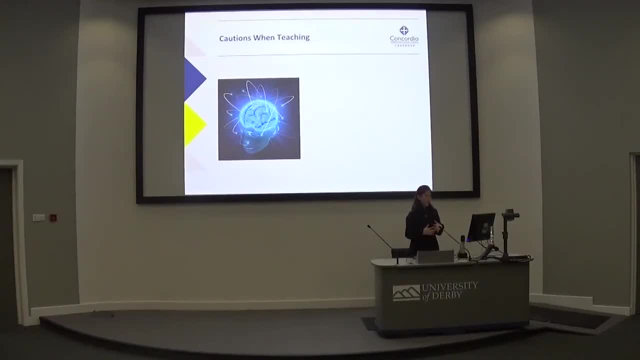 and cherish our human qualities, such as our emotions, our intuitions. And also. the teacher will be stressing about the importance of proper interpretation, How proper interpretation should be used, how proper interpretation should not be biased. It should be objective and proper interpretation. 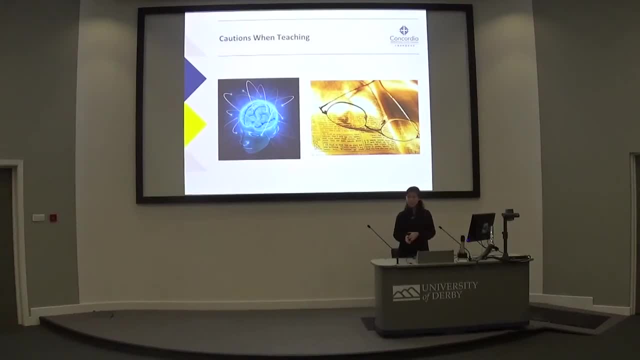 by a subject matter expert and essential here. The expected outcome of this course is going to be concluding in three words: Exposure, application and awareness. By the end of the course, the students are expected to be well-versed about big data. 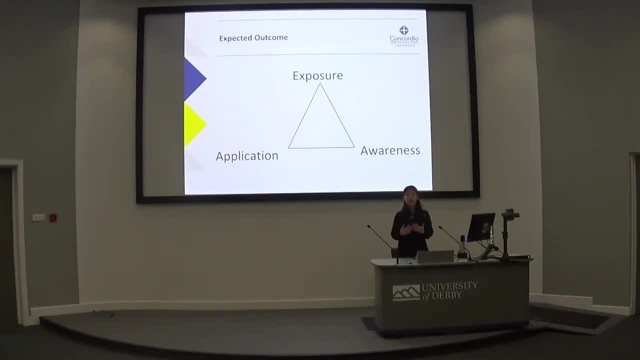 They will know, they can explain to others what is big data, how is it used in life and also the benefits or the dangers of big data. And also they will know what is going on there outside of their school and just learning, what is the trend in the world too. 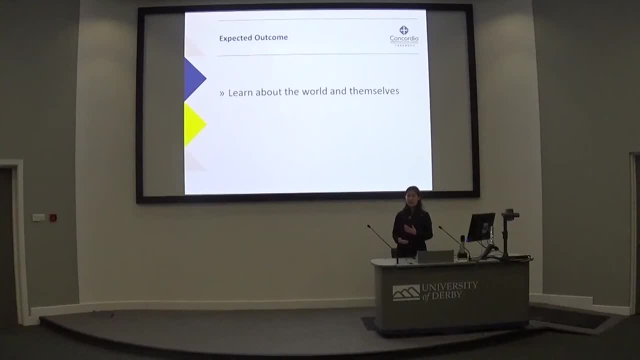 They will learn about the world and themselves as they work on the projects, their own directed projects, And they will also be more enthusiastic in learning because they know that the knowledge they're learning right now is relevant and it is right now happening in their lives.